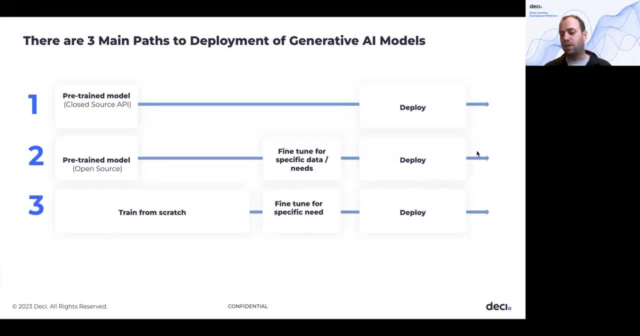 then deploying it in their premise, in their cloud or in one of their services, like SageMaker or others, to serve those models. So that's the first step. The second step is to build a model from scratch, And the last, and the more complex one, is to train from scratch. and this is really 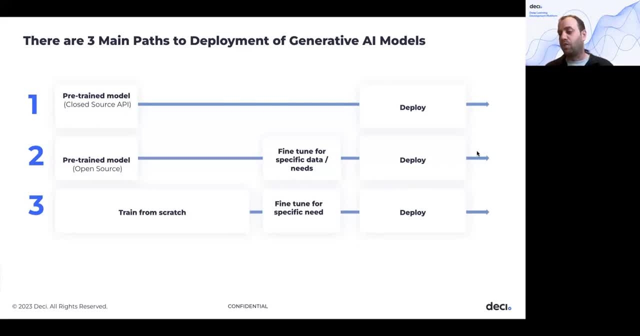 being done, and this is done especially when there is a domain shift or a different domain that we need to build models for, such as financial aspects or healthcare or other domains that requires a different pre-training, other languages and things like that. So, basically, those are the three paths. 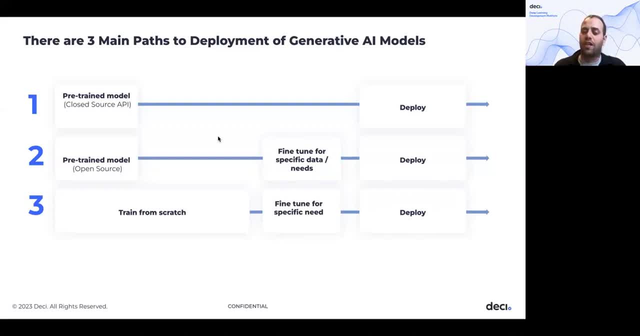 that at the end we are getting to build models and then we are going to go ahead and build models. So having a model in production- but having a model in production- is only the beginning of the journey in that essence, because we need also to build the application around that model, We'll 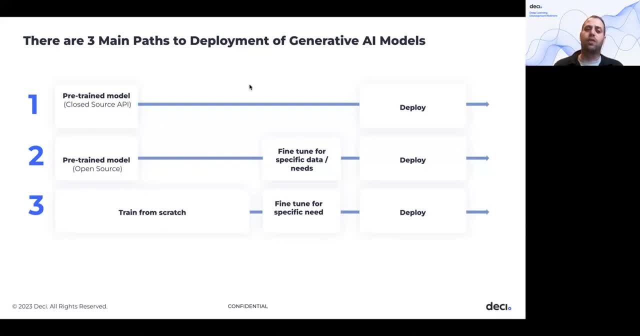 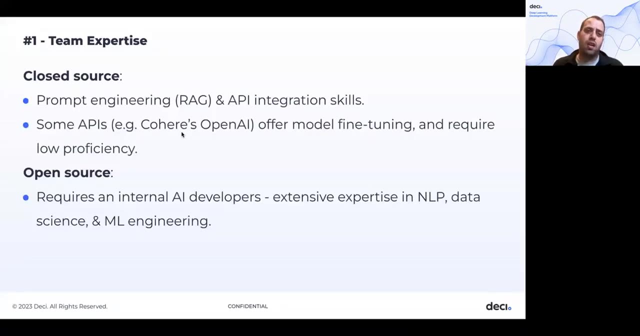 talk about all of these and what are the pros and the cons of going closed source versus open source in the journey to get models working for us in production. So we'll talk about some of the consideration and we'll start with the required team expertise in order to build based on closed source or open source. 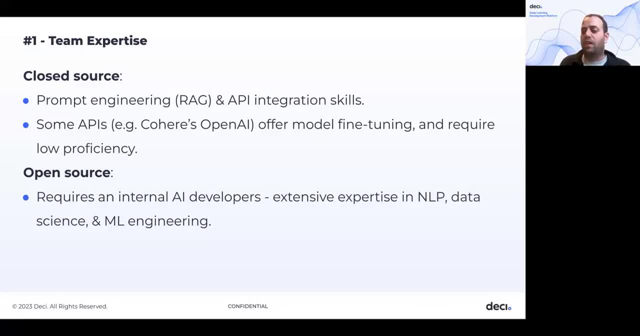 So when we're talking on closed source is basically integrating an API, So it's a software development skills. even if you're using things like RAG, retrieval, augmented generation or things like that, that's relatively easy integration to use closed source models that are given through API. 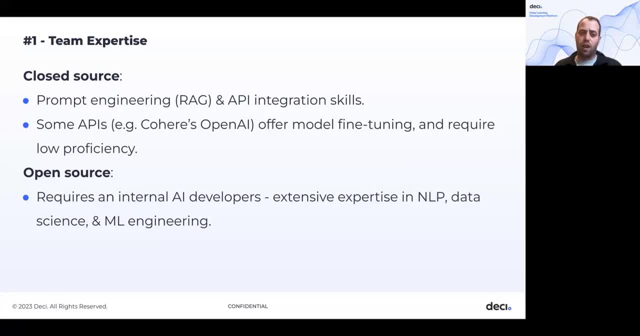 with documentation and examples. So APIs like Cohuse and OpenAI offer model fine tuning and require low, low proficiency because this also streamlines through API calls. In open source it's a little bit more complex and require the team to choose the right model, to fine tune and customize it and then to deploy it on on their 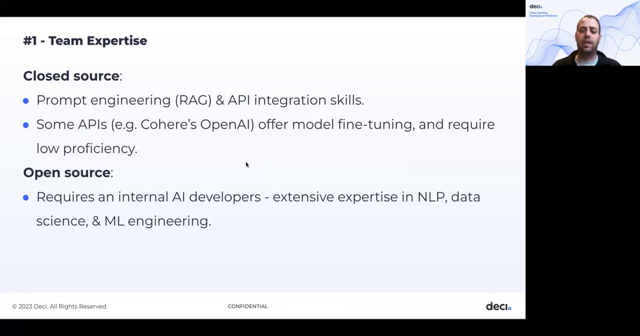 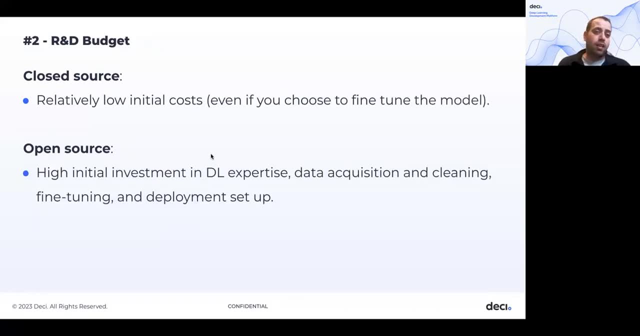 cloud and maintain like high availability and and things like that, which make things a little bit more complex in the journey. And the second thing that we have to that is highly correlated with the previous bullet- is the R&D budget, So there's low initial costs when we're going closed source. Basically, we just need to subscribe. 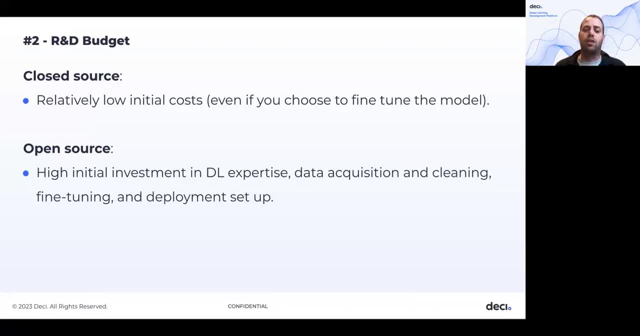 to one of those services and integrate the API. and when we're going open source, we have to get the expertise to the team to acquire some data, to do the fine tuning and to deploy the models in case that we're going with the longer journey, And that's the reason why we need to have a good historical-ionen of customizing the open source models. 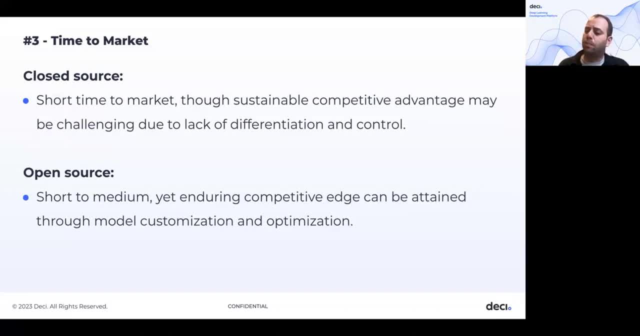 Also the time to market. Obviously, integrating API is quite easy, So at least for the POC level to get a demo up and running. connecting to an API gets us to something very fast, but later on, when we're trying to build something that is more customized, it will be a little bit harder on the closed source. 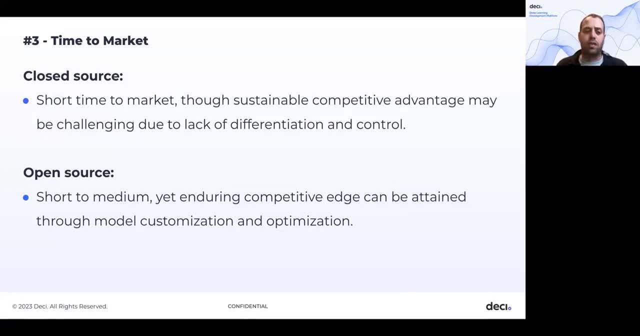 models, cuz, cuz. it's hard to, in most cases, to customize them In open source. it will take a little bit more time to get something that is working, but the ability to customize and optimize later on is easier. So on the short term, 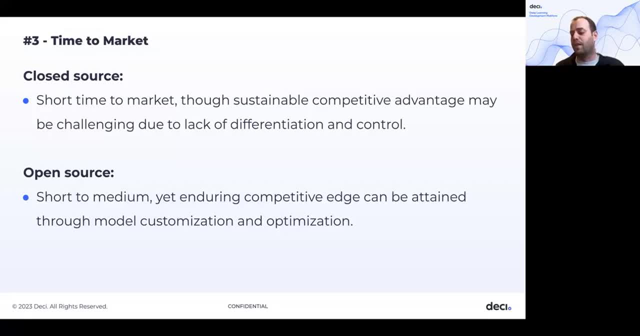 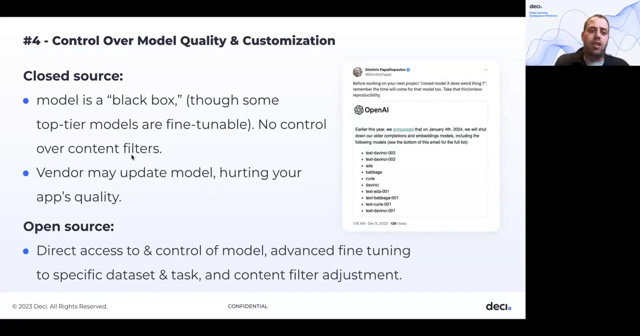 the time to market is faster on closed source, but to get really up and running with what we're looking for, which is a customized Gen AI model, will probably open source will be a competitive option In terms of model quality and customization. in closed source, the model is a black box. 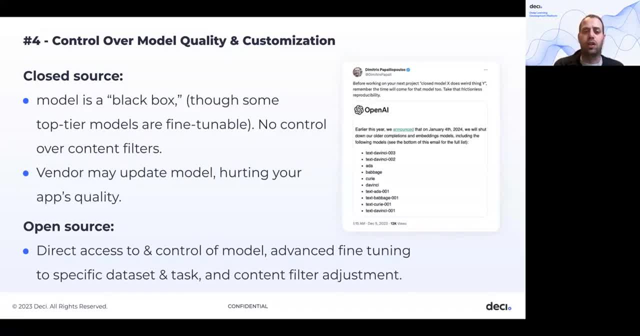 We don't know even what is the size of the model. for most of the model We don't have control over content filters that those vendors are putting on the model And vendor may update the model, which is something that might change the quality of your application. 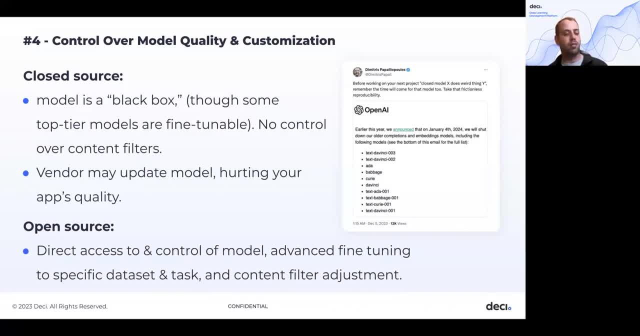 And also they will retire some models and get some models, some new models out. And this is an example for a past form this week, showing that open AI show that they will shut down some of the older models they're having in an artist of one month. 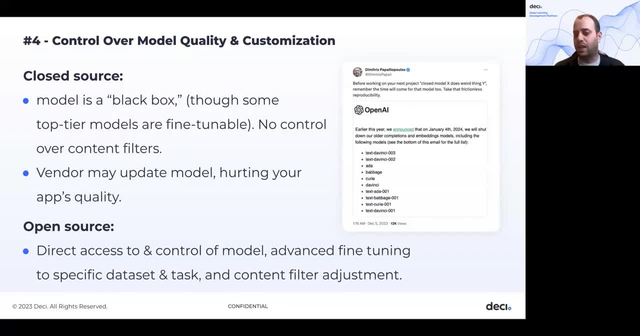 or something like that. So if you build an application around that, you will no longer have access to those models and you need to change your app. So you need to do that again, like build on top of newer models and things like that. 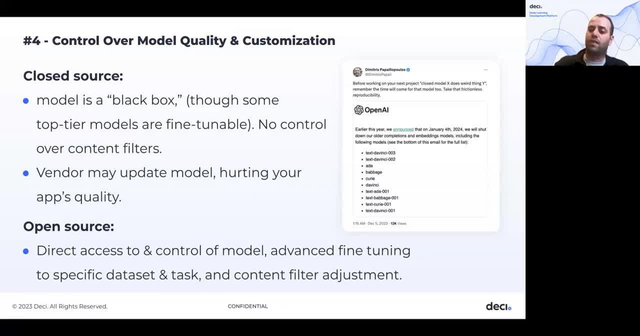 And if you're using a vector database with some embeddings that you built on some of those models, then you'll need to map your entire DB based on a new model. So replacing a model is not something that is very easy in some cases And you don't have control. 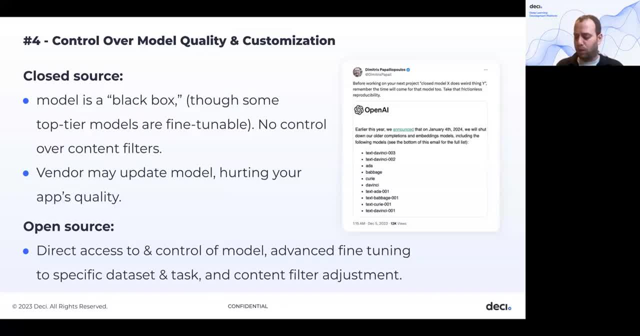 when the vendor that's selling you the model will choose to shut down the model and get you updated to a new model, And that will probably hit you in one month's notice and will require you some R&D effort. So this is just a real example from this week. 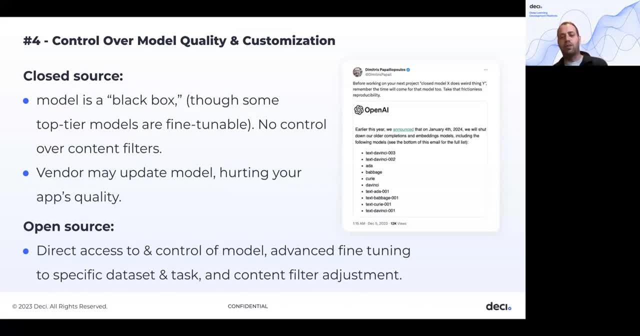 In open source. you have full control, access to the model. You can fine tune with various techniques- Either it could be reinforcement learning or QLore and things like that- And you have more control, no content filters, So you can. 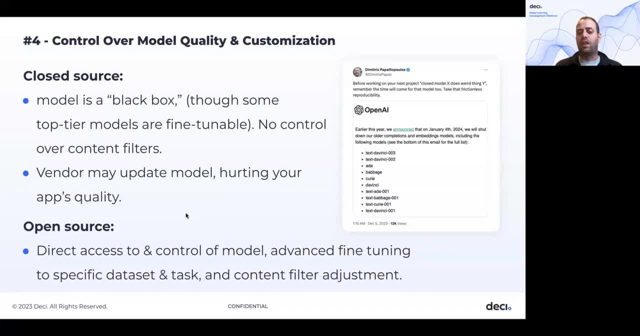 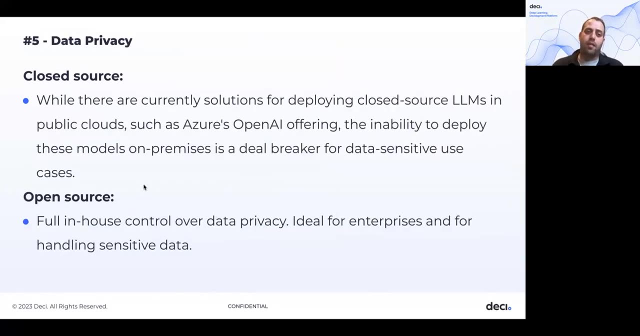 Build your own content filter or safety nets and things like that, And you simply have more control over model quality and over the model itself, basically, and how you run it. In terms of data privacy, most of the closed models are given through API. 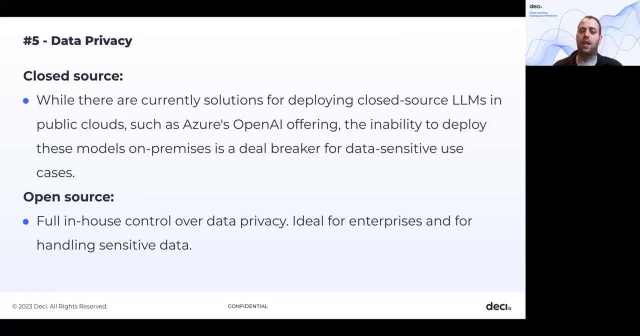 which is outside your cloud solution. In some cases we see companies like Azure, OpenAI, joint, offering that you can take open AI models into your VPC, But in most cases it will be challenging to use closed source models without sharing the data at inference time. 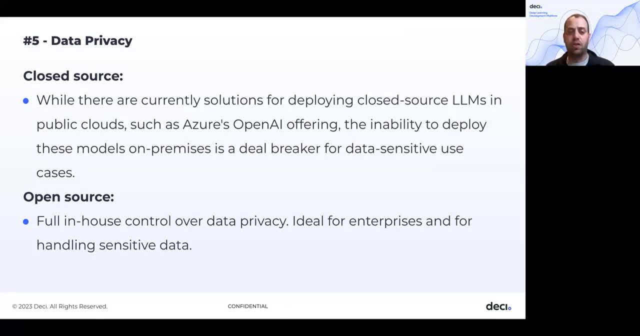 with those solution provider. On the other hand, on open source, you have full control on where the model is running, So you can basically run it in your VPC, And that's ideal for enterprises handling sensitive data, such as healthcare companies. 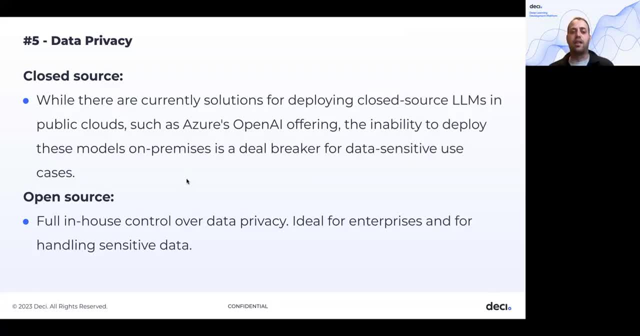 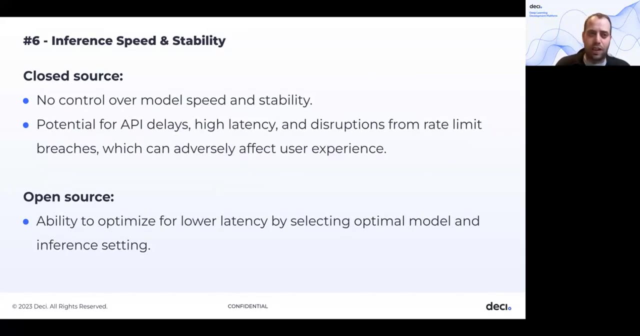 and financial services company that the data privacy is very, very important on those areas, for example. So data privacy is an issue. Last thing is inference speed and one before the last is inference speed and stability. So on the closed source, you don't have any control over model speed and stability. 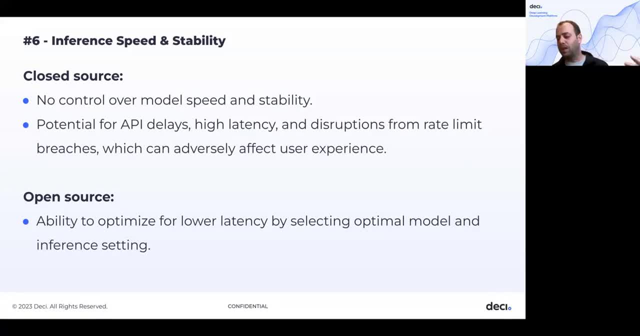 Obviously, those model providers are having their own demand and they are making a lot of money and they are managing batch sizes and the queues and the scalability of the workload. So you don't have any control on how much you will be queued and in what batch size the workload will work. 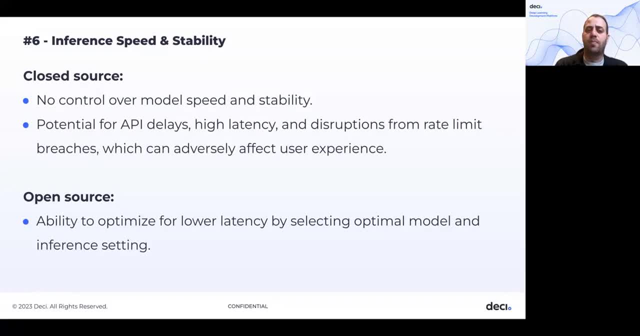 So basically means how much you will wait and what will be your latency, And you are up to their settings in how good your latency will be. Also, API delays due to high load and, at some hours, high latency and disruption in services is something. 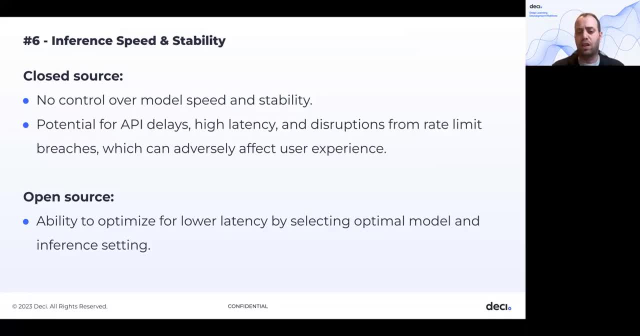 that can affect user experience in your application. On the other hand, open source will be more effort to put up in production, but you can optimize the latency- which is something that we will talk later on- and choose the optimal inference setting for your need. 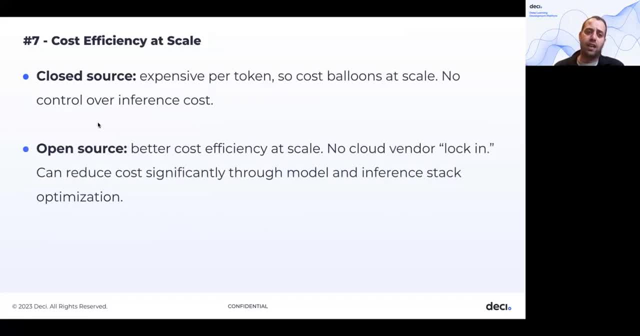 Last thing is the cost efficiency at scale. So basically, in closed source you're paying per token With high, relatively high cost per token. that scales linearly when you're going to scale And in open source, maybe the effort to put it up. 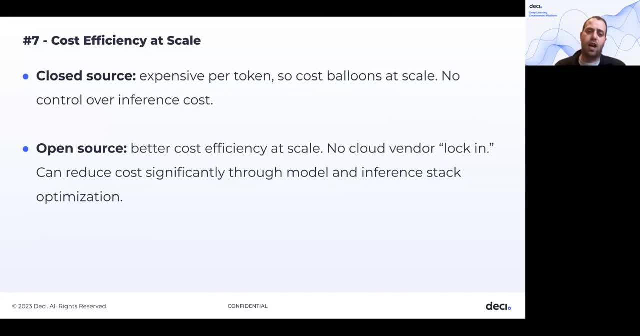 and running at the beginning is higher, as we referred in the R&D cost, but the efficiency or the price that you're paying for token is significantly lower, And we'll see that in a second. because of that, you can choose a model that better fits your app. 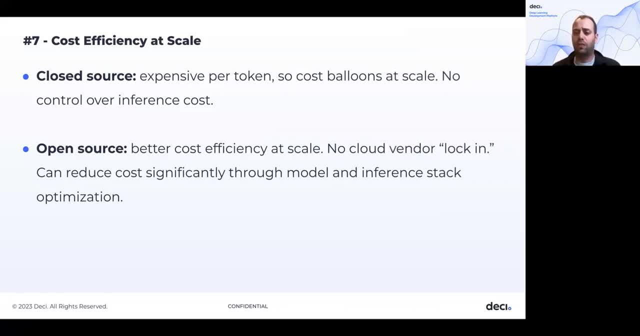 You don't need to go to GPT-4.. You can use a 7 billion parameters for some of the use cases that you are building And those are running much faster and in much better performance and cost compared to the very large models. 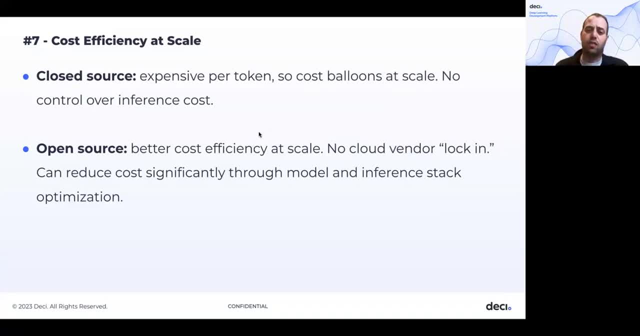 You can also go to 70 billion models and things like that. So basically you have to control over the size of the model, which basically also give you control over the latency, over the cost and over the throughput of the infrastructure that you're running. 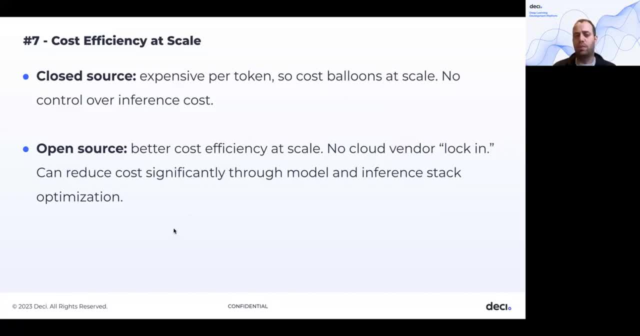 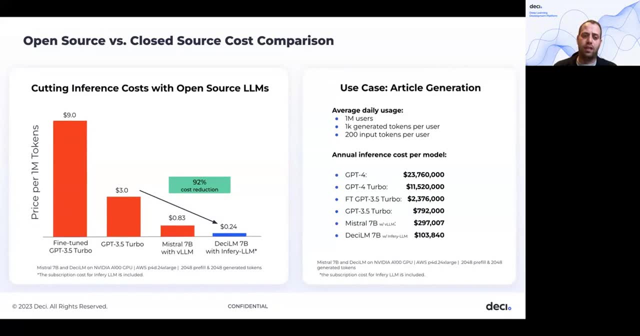 In order to run those models which you can optimize cost and efficiency. If we compare the open source versus closed source pricing, here's an example for a 7 billion models like Mistral and SCLM- that we'll talk about it later- compared to GPT 3.5 Turbo, which is a bit larger. 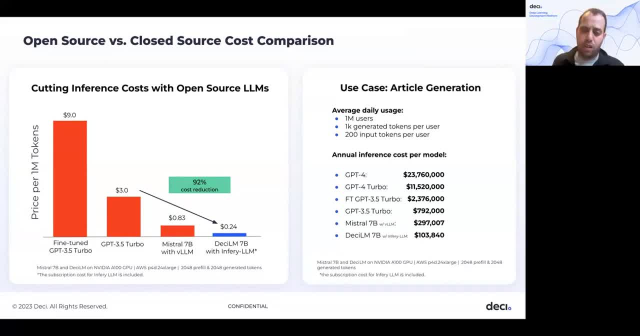 And in some cases have better accuracy. but in many cases you can use 7 billion parameters model fine-tuned in order to replace GPT 3.5 Turbo And what we see here is that is something like 92% cost reduction when considering moving from GPT 3.5 Turbo. 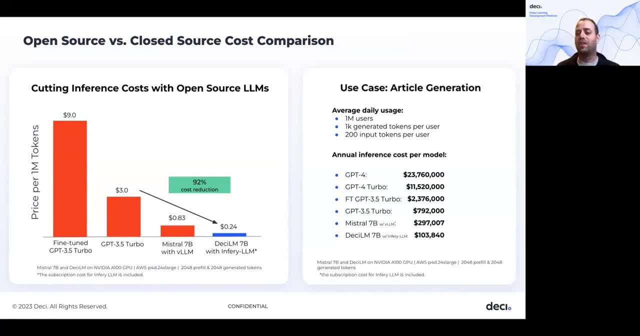 which is considered one of the cheapest closed source models available, order to run open source models on your existing stack with some level of optimization, such as VLLM or InferiLLM. that we'll talk about it in a second, And here's on the right. 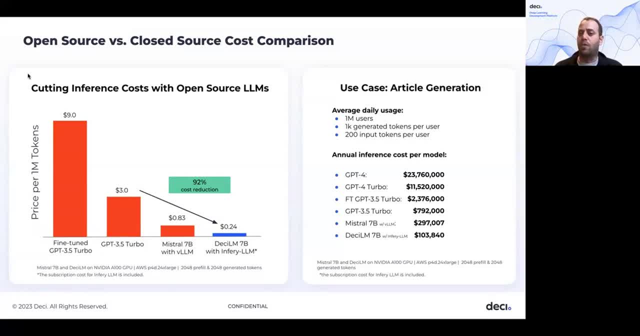 you can see a use case example of 1 million users that generating 1K token per users with relatively short context or short input tokens And you can see what will be the cost of running that scale on GPT-4, GPT-4 Turbo. 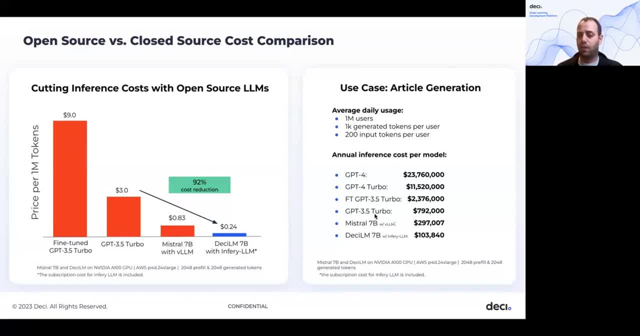 fine-tuned GPT-3.5 Turbo. GPT-3.5 Turbo without fine-tuning, Mistral-7b with VLLM, which is an inference engine in open source, and Desi-LM-7b within InferiLLM. 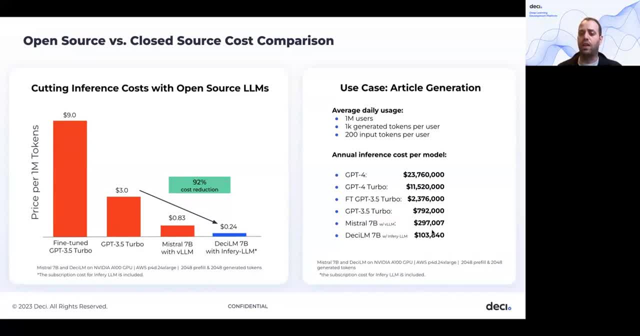 which also encapsulate the cost of InferiLLM, which is part of Desi's commercial offering. So what we can see here? that the cost reduction is massive. Obviously, we cannot compare GPT-4 accuracy to Mistral-7b. 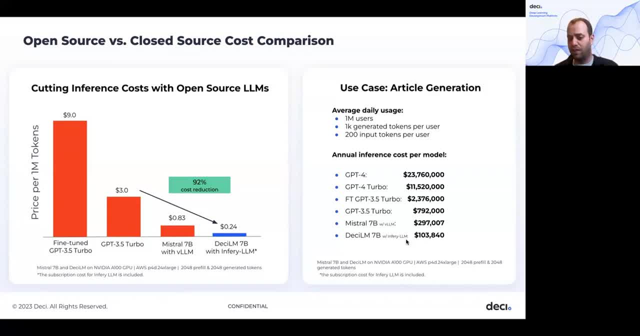 but that's really really depends on the application And we can assume that the cost of serving a 70 billion parameters model or 30 billion parameters model will be somewhat in the range of the 7b multiplied by some factor and will still be significantly. 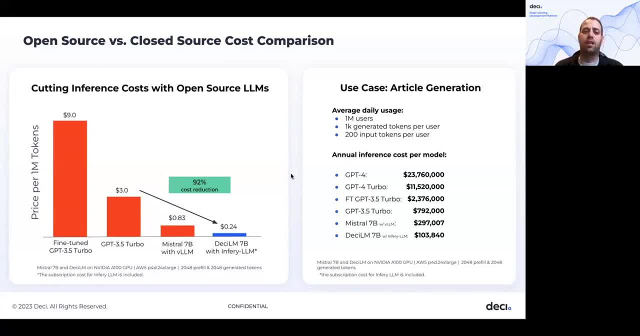 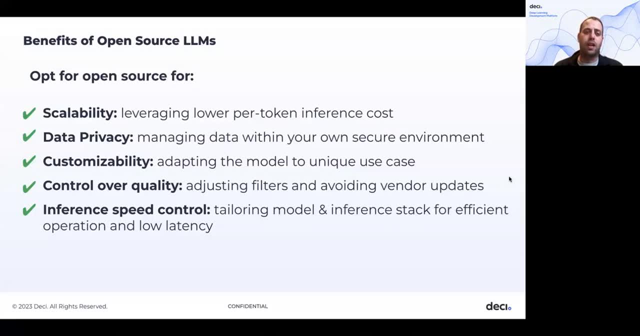 very significantly lower compared to the closed source alternatives. So, if we think about the benefits of going with open source- the scalability that we just saw, scalability that we just mentioned, the data privacy that we mentioned earlier, the ability to customize the model and control over the model quality- 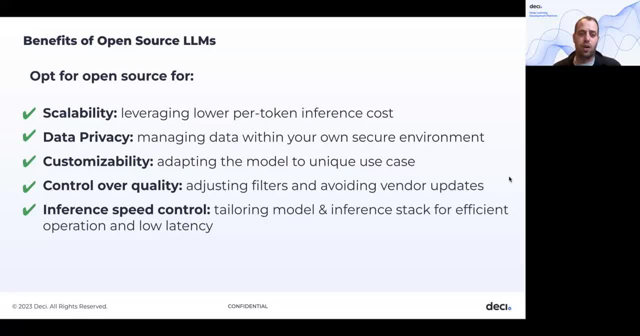 and control over the behavior of the model And, at the end, the inference speed, tailoring the model and the inference setting to operate in low latency, for example, or in high throughput, based on your needs for your applications. So those are the benefits of using open source. 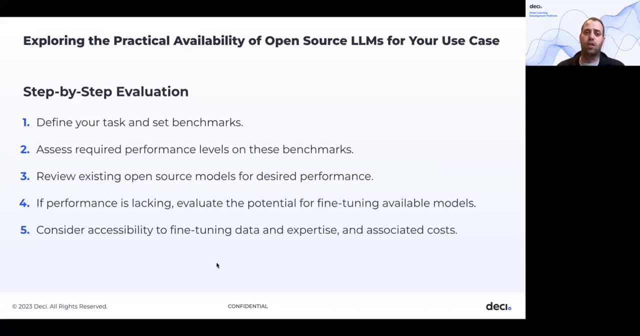 More of those compared to the closed source. So where to start? If you want to start play with open source model, first thing to do is to define your task and set how you want to measure yourself. then see how you can get the required performance. 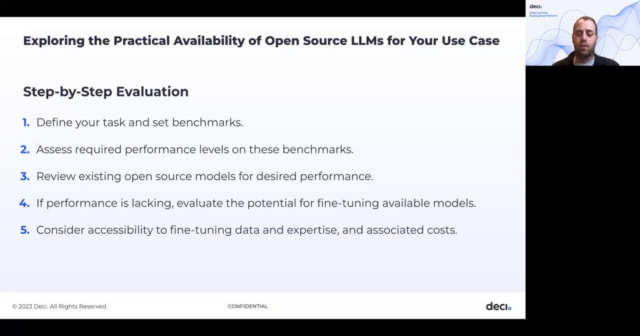 on these benchmarks either, using some starting with small open source models, fine tune them, test them on the test that you want, test them on the test that you want. review some examples- And there are many examples in open source- on models that have been customized to specific use case. 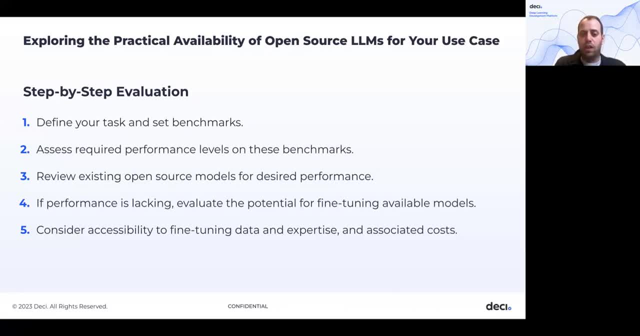 and then consider fine tuning, collecting data and improving the fine tuning techniques. We see a lot of new techniques to fine tune with reinforcement learning, LoRa, QLoRa and others, So you should explore all of those and also hyperparameter search and many things to improve. 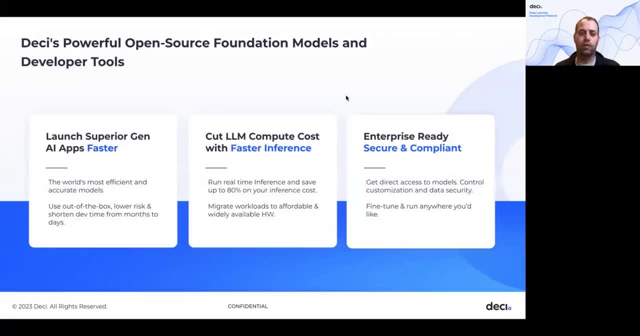 fine tuning to get your model to the level that you're looking for. So what is DESI and how it is all related? DESI has open source foundation models that you can find on HuggingFace and we'll have some links later on. 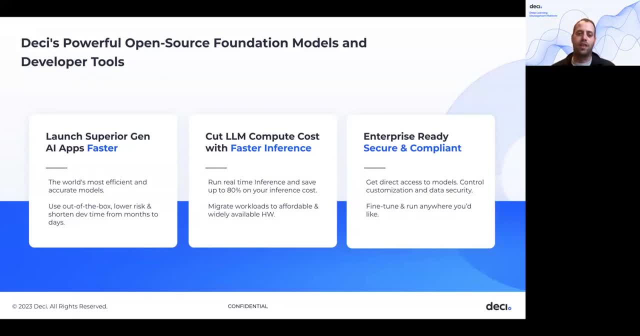 And we are also launching new models very soon, So we'll expose some of their capabilities in these slides. But DESI enable companies to launch superior gen AI applications faster because of using models that are better, and we'll go through those models later on. 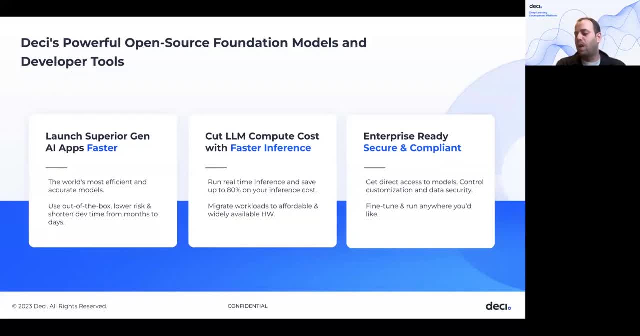 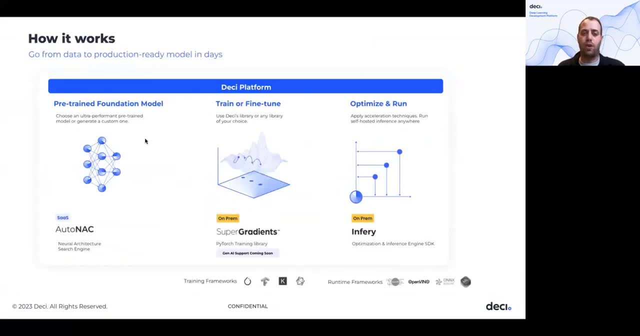 Cut the LLM, compute costs with faster inference and do everything in your premise in a secure and compliant way How it works. So we have a pre-trained foundation model families that some of them appears on HuggingFace- The option to fine tune them with our libraries. 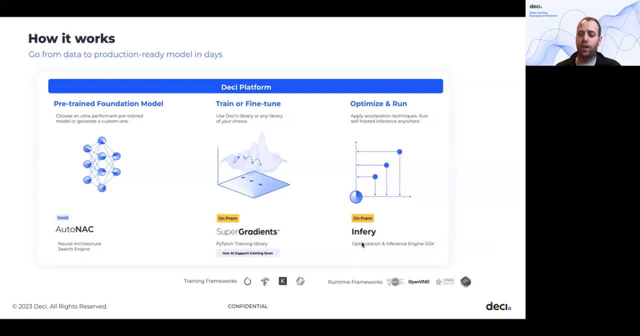 and optimize and run them with an SDK that is called Inferi, which is basically optimize those models to production and run them with all the best of breed of techniques, including CUDA kernels and things that we developed in-house in order to make those models run really, really fast and efficient on GPUs. 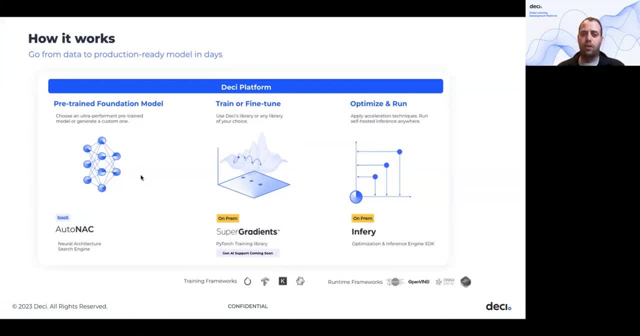 The core technology of DESI resides in how we build those foundation models to be more efficient, And I will show some of those models and examples in the next slide. But the idea is we use technology that we call Autonac, which is coming from the family. 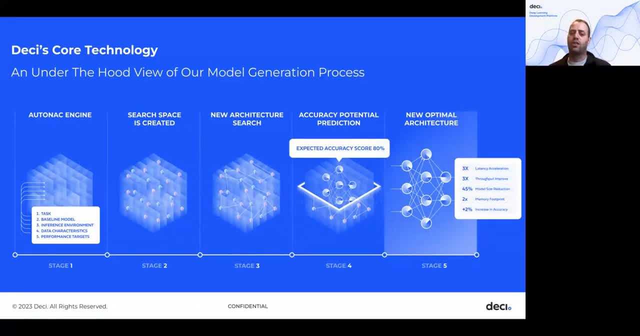 of neural architecture. search, that basically choose the best model out of trillions of candidates, which is, those candidates resides in something that we call the search space. We're searching for the best models out of that search space And at the end, we end up with new architecture. 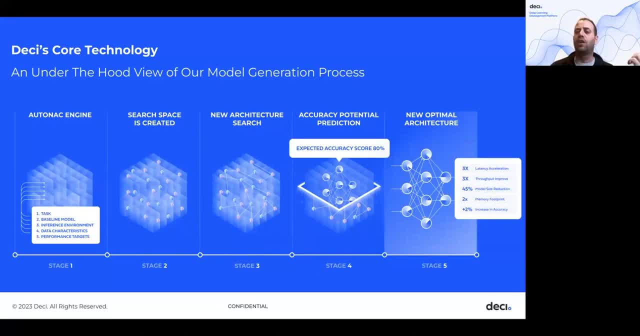 that meets, on performance, our criterias that we are looking for, And then we train those models. So we started with that technology for the computer vision models that we also released in open source models, such as YOLO, NAS and some other models. 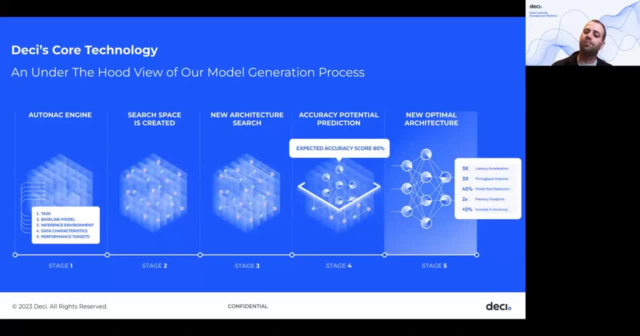 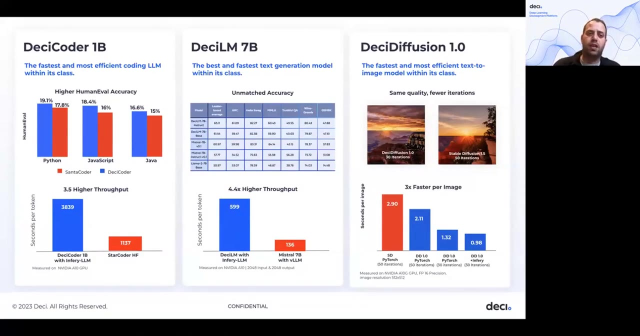 for other tasks, And then we built a couple of foundation models in the text to image space and LLMs that we'll see now. So the first model that we released was Desiccoder 1B. It's a very efficient code generation model. 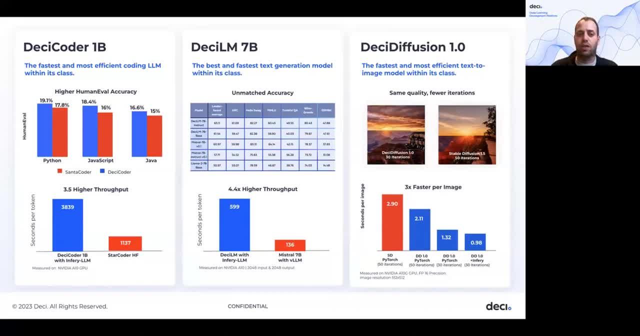 which is competitive to Santa Coder, which is a 1.1 billion parameters model, And the idea here is to build a very efficient model that can run very fast, with good accuracy compared to that Santa Coder that we can see here. So that model is available on a hugging face. 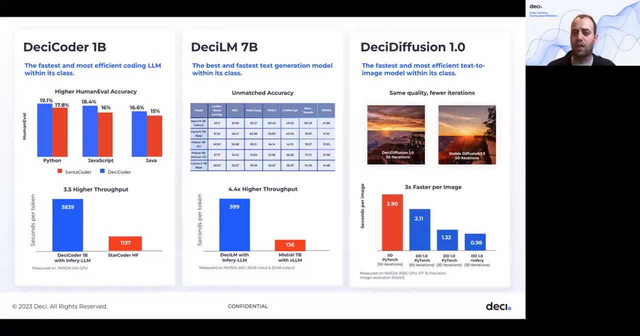 We see a lot of trends. We see a lot of construction for that model in terms of number of downloads and things like that. It's a very permissive license. The next model that I will talk about is the CLM 7B. 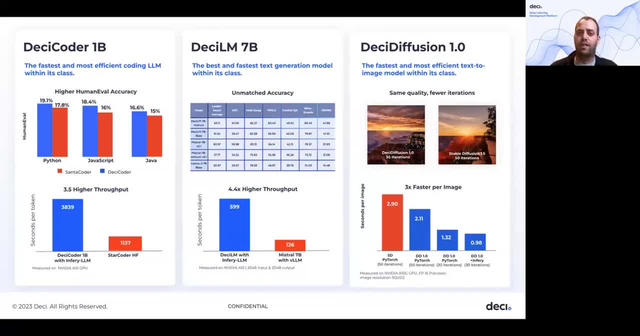 This is a pre-released version of the CLM, which will be released very soon, But I'm exposing here, I think for the first time, the numbers that we've got. So the CLM came to win the 7 billion parameters model. 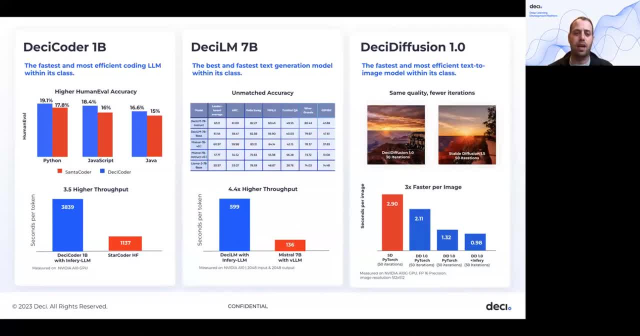 cutting edge. So the CLM is a 7B category which currently dominated by Mistrel 7B and Llama 2.7B And it outperforms those two models. We have a base model version which you can see the numbers here. 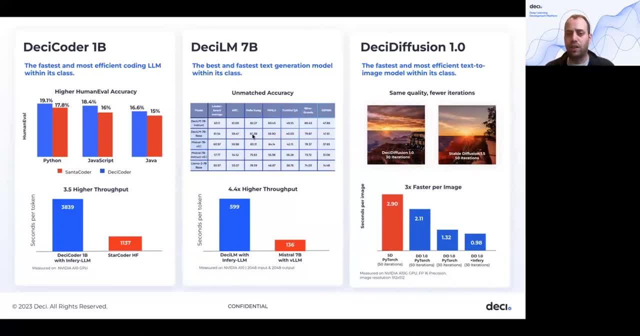 on what is called LLM open leaderboard- open LLM leaderboard and an instruct model that is slightly better. So if we compare all the base models in that leaderboard, I think that the CLM is going to be the first one out there. 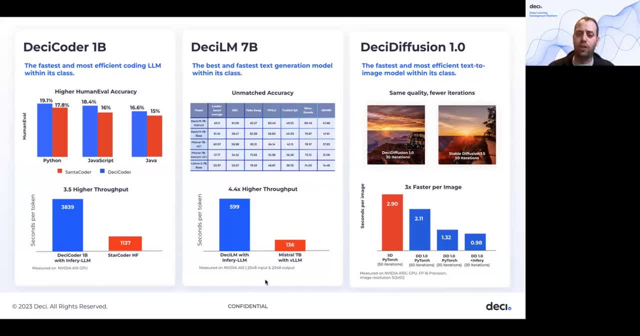 But it's not only more accurate but also more efficient or running in higher throughput. And what we can see is that when you take that model- and it will be an open source very soon- And when you take that model and running it in its open source version, 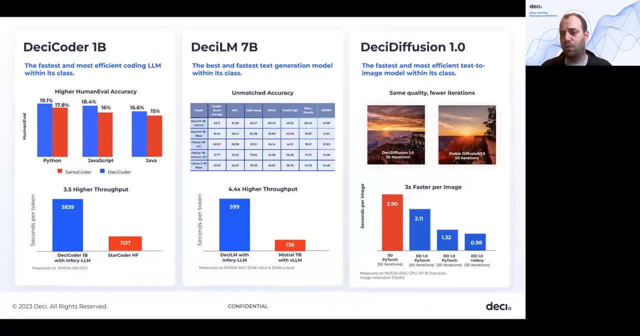 what you see is that you can get something like up to 2X improvement in throughput. But when you bundle that model with DESI's inference engine that I will present in a second, you can get up to 4.4X higher throughput. 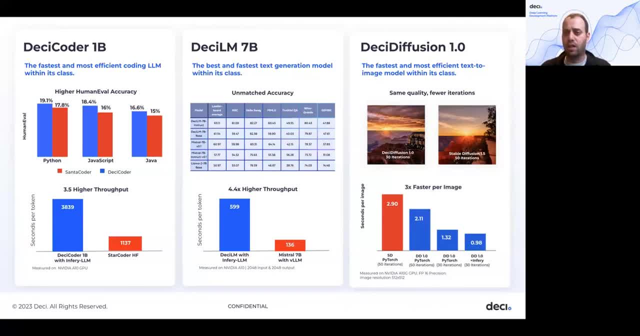 which is very important for reducing the cost and reducing the latency of those models running in production. Another model that we released is DESI Diffusion. DESI Diffusion is a text-to-image model that is similar in its performance, in its accuracy, to Stable Diffusion 1.5.. 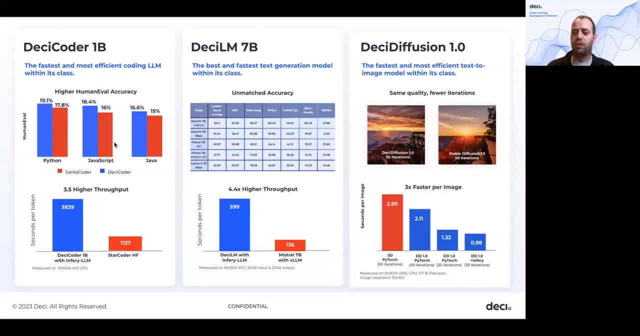 It's running in fewer iterations compared to Stable Diffusion And it's running 3X faster per image. So when you're running on NVIDIA A10 GPU, you're getting an image by less than one second, which is what we aim for. 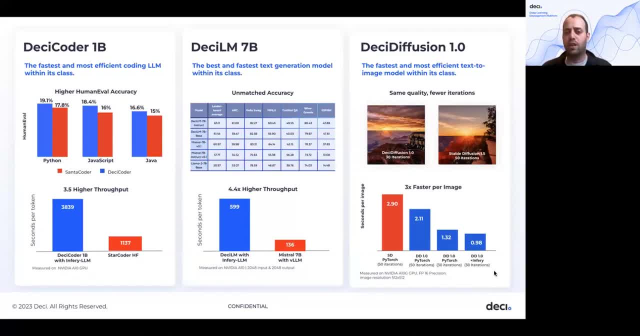 Obviously to the data, like in the couple of last weeks, they were introduced a lot of techniques to reduce the amount of iterability, to reduce the amount of iteration, distillation and things like that. So we are working on those as well. 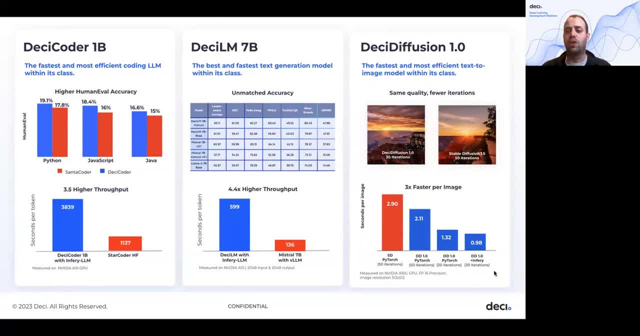 And we'll probably release a new text-to-image model soon with better performance than what you can see here. But currently, if you're using Stable Diffusion, you can simply switch to that open-source version of DESI Diffusion that appears on HuggingFace. 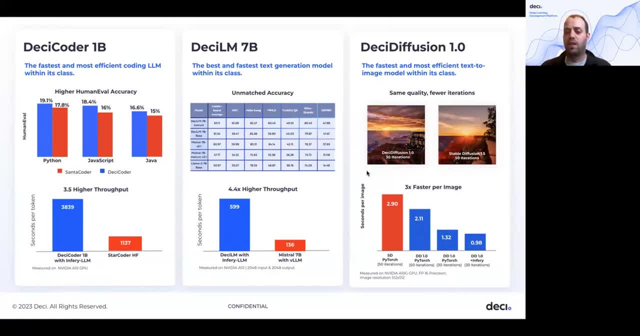 that's giving a significantly better performance and also reduce the amount of iteration to get the same quality. So what we're doing is we're going to use DESI Diffusion 1.5.. So we can see here that PyTorch versus PyTorch. 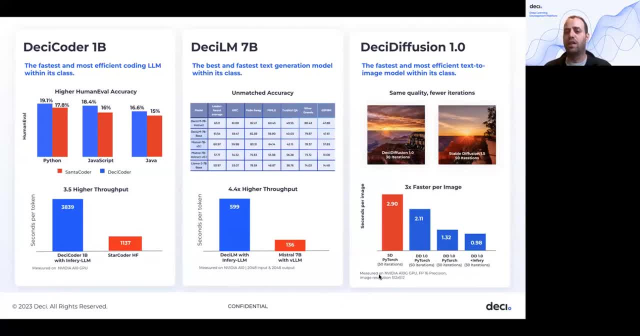 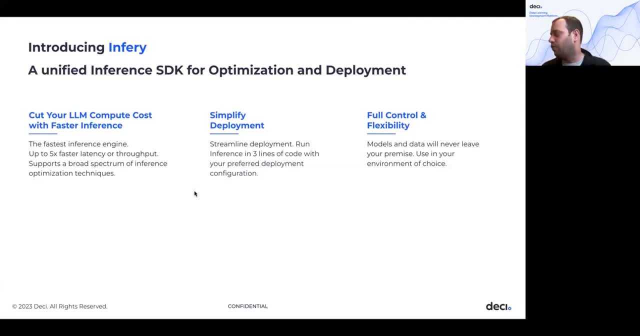 you're getting more than 2x improvement when using DESI Diffusion compared to using Stable Diffusion 1.5.. I talked about Inferi, which is DESI's runtime engine for inference, So that's an SDK that our customers are taking. 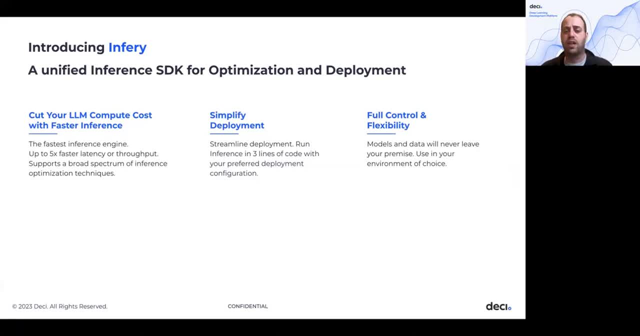 to run in their environment, And Inferi is helping with squeezing the maximum out of the available compute. So it usually works with GPU, but it supports a few other hardware types And it's reducing the cost. It's simplified the deployment and it's giving control over the deployment. 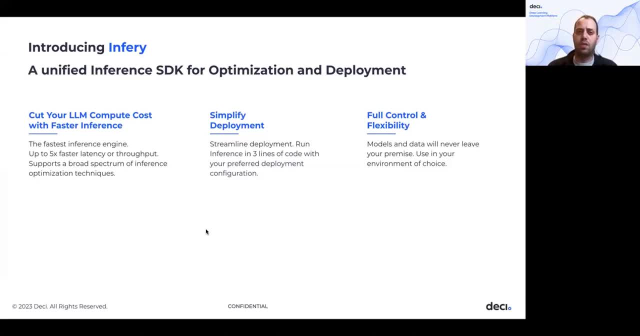 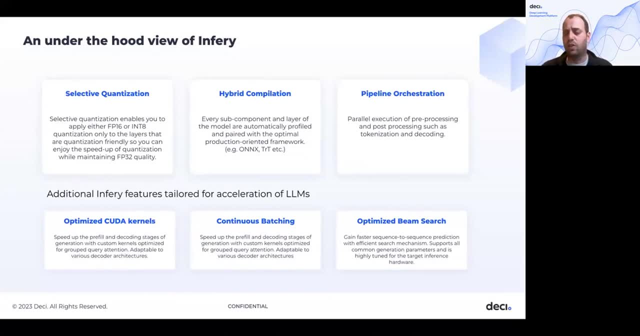 in terms of performance and trade-offs that you can calibrate when running the models. Under the hood of Inferi's LLM version is several techniques in order to improve the efficiency and the performance of the model. So Inferi LLM supports selective quantization. 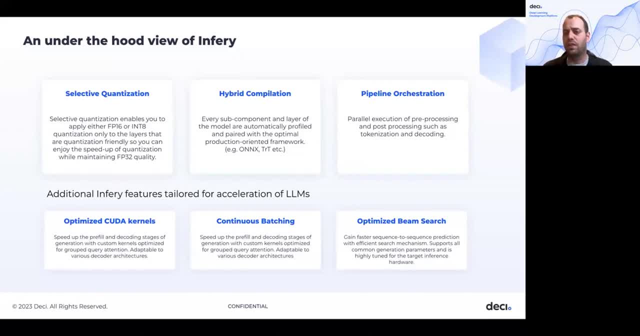 which basically takes different layers to different quantization level. that helps manage the trade-off between quantization, like performance, and accuracy, that is, in accuracy degradation. that is sometimes happening due to quantization. Hybrid compilation: some components can compile, some components cannot compile. 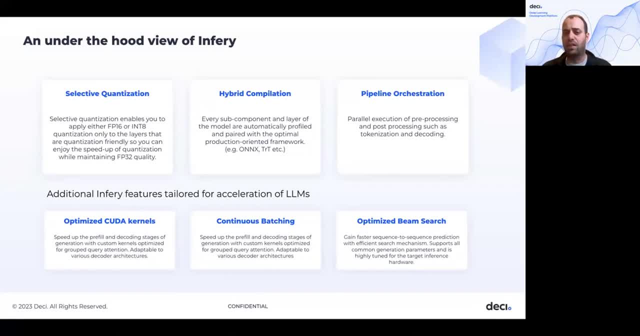 So we are kind of mixing some techniques and frameworks in order to, you know, to compile complex models within Inferi. Also, pipeline orchestration, parallelism over the pipeline, for example in LLMs doing the tokenization in parallel to doing the inference, and things like that. 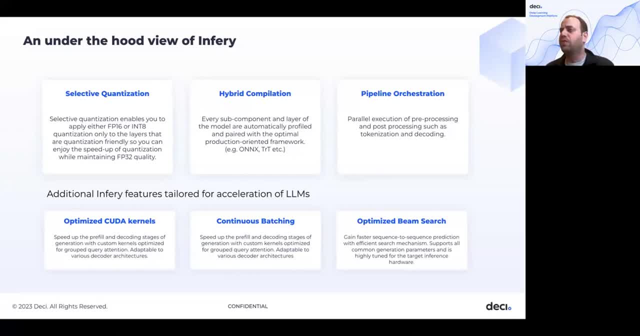 And where the performance boost is coming from. first of all, Inferi LLM is built to serve Desi's model, So Desi's architecture, that generated by Autonac, optimized to run on Inferi LLM and to run with the underlying hardware. 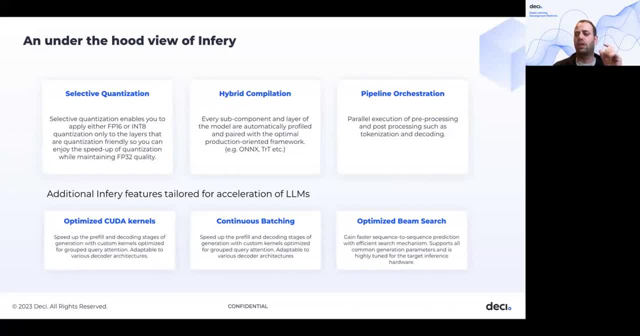 So Inferi LLM has optimized CUDA kernels to run the models built by Desi in a way that is improving the performance of Desi's model with the appropriate CUDA kernels to boost the maximum performance. We did a lot of optimization in the lower level of CUDA. 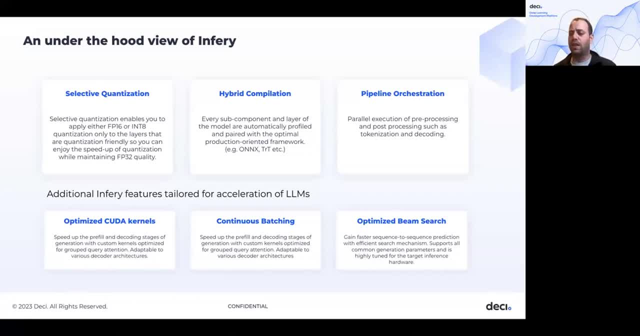 Another thing is continuous batching. Continuous batching is the ability to run in-flight batching, send multiple requests and aggregate the batch, which you can add new requests to existing batch and pop out completed sequences out of the batch and make space for new requests. that's coming to. 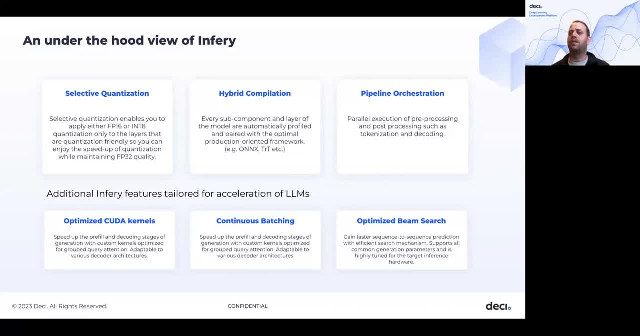 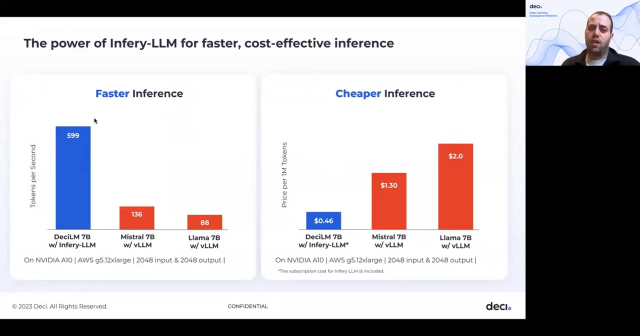 the server. So that approach, helping to optimize the workload from a server perspective and optimize sampling, such as beam search and standard sampling, is also one of the features that enabling us to push the performance significantly for models that are running on Inferi LLM. So the power of Inferi LLM when bundled with this model is improving the tokens. 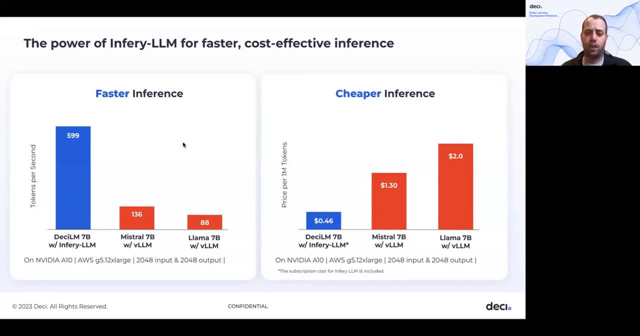 per second, Basically the throughput of the models. if we see here Lama 7b and Mistral 7b when running on Inferi LLM, the power of Inferi LLM is improving the tokens per second. So the power of Inferi LLM when bundled with this model is improving the tokens per second. 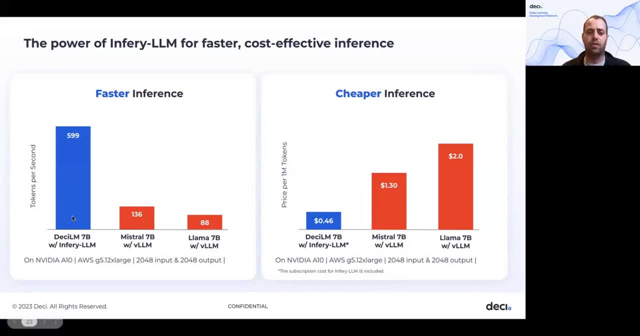 So the power of Inferi LLM when running with VLM, which is a leading inference engine in open. So what we can see is that Inferi LLM, when bundled with this LLM 7b, is improving in a factor: the throughput of those models, And obviously throughput is translating. 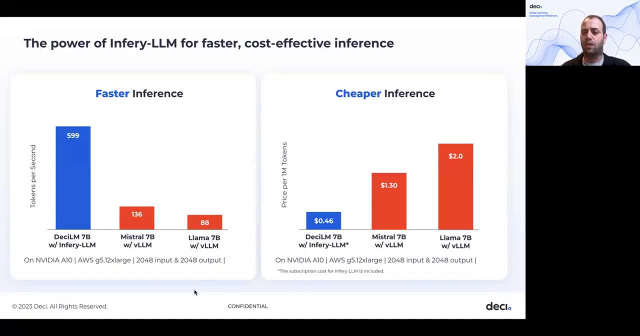 immediately into cost And we can see the same factor that is being reduced significantly in cost of serving, And the numbers here are a calculation of 1 million per token, which also including the subscription for inferior cost. so this is the real net cost reduction that you're seeing when you're using inferior length for for those things we're working. 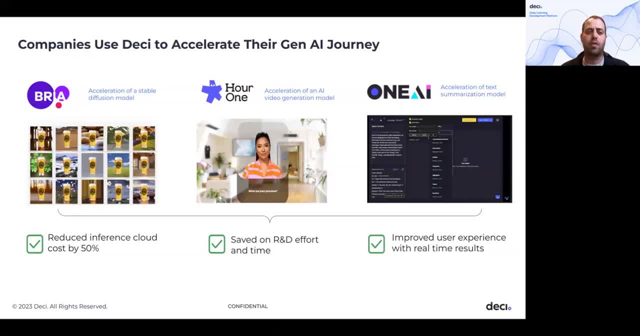 with many companies in the gen ai space. some of those that i can share are doing text to image for visual ai platform, avatar generation in videos and and text nlp platforms, and we are having more and more companies using desi open source models that obviously we don't know. 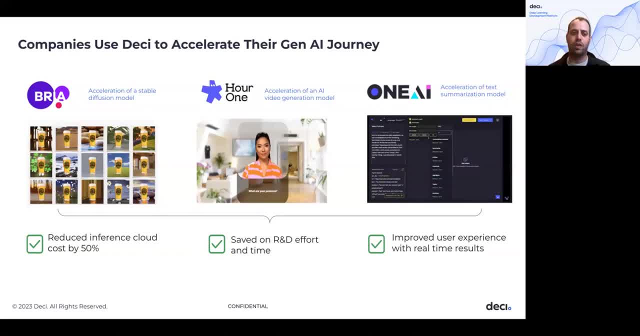 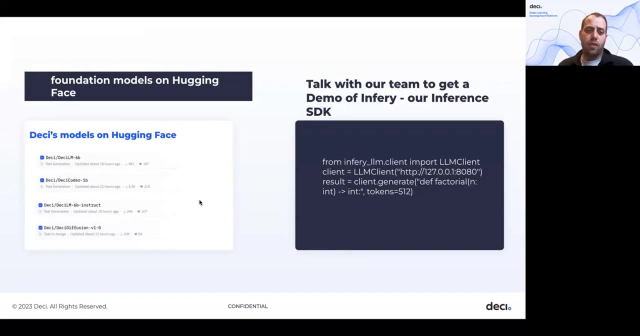 anyone, everyone that's using those models in open source, but they have a very nice traction, and also companies that using in furry to run those models in production, both for computer vision, text to the image, models and llms. if you want to test those models, those are the models. 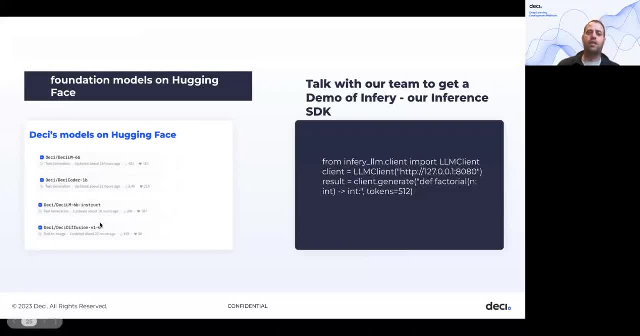 that currently are listed on on this is hugging face um account. uh, so you can try. what we can see is the clm6b. i promise that soon we'll we'll have a 7b version over there. the clm6b is the previous generation, uh, desicoder 1b that i. 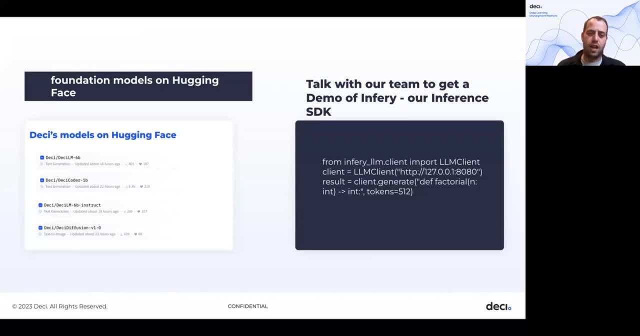 mentioned um the clm6b instruct and desi diffusion, which is the text to image model uh that i mentioned earlier. also, we you can talk to our team through our website in order to get a demo of what the lms boost looks like and how you can start using inferior lm in a very simple sdk. 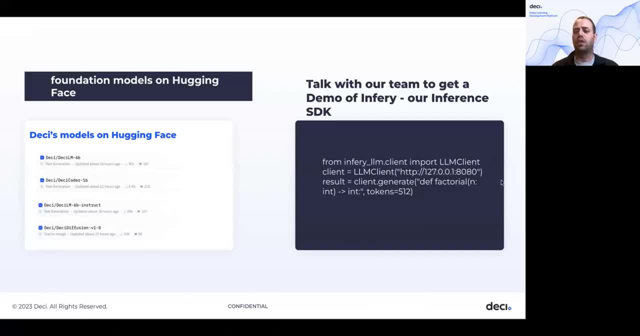 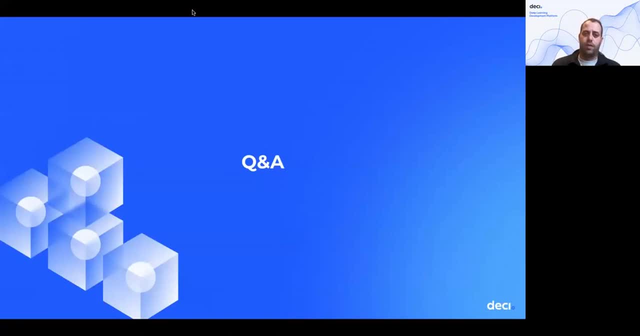 installation on your premise, replacing the tools that you are currently using in order to to run llms or other models in production. we'll move to the um, to the questions. uh, let me see and open all the questions um. so the first question is, and the easier to answer is, whether the, the, the. 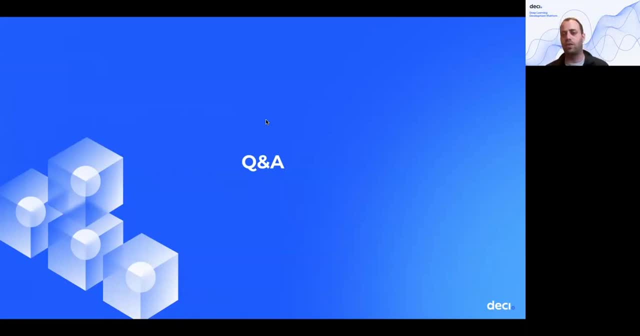 um, recording is going to be released. uh, yes, so you'll get a follow-up email for all of those who registered to that webinar. uh, with the recording. uh, so some question. uh, so, in terms of uh model loader you use for this code and what is the prompt template? so we have examples in the in the model. 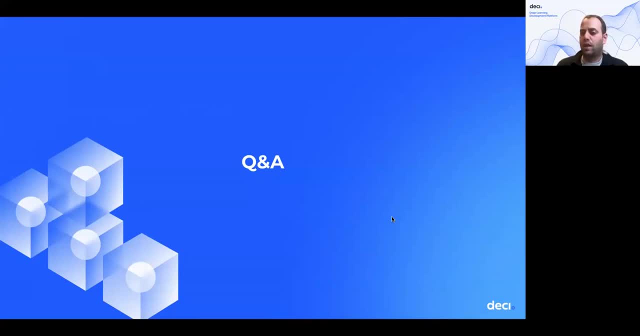 call or hugging phase uh for the instruct model and and the instruct um prompt template that you can use. and if you have any more questions on specific um how to use the instruct model, you can uh open an issue in the in the community page in the hugging face repo of uh the model. 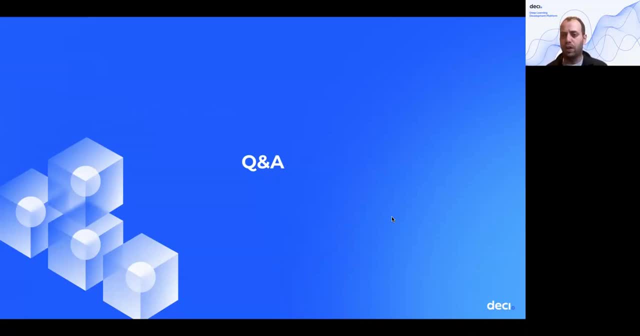 the next question is how to perform compared comparison between open source versus non-so non-open source llm and what benchmark can be used. so, generally speaking, quality evaluation of lms. um is a is a is a open question, uh, and it's really hard to to find the one size fits. 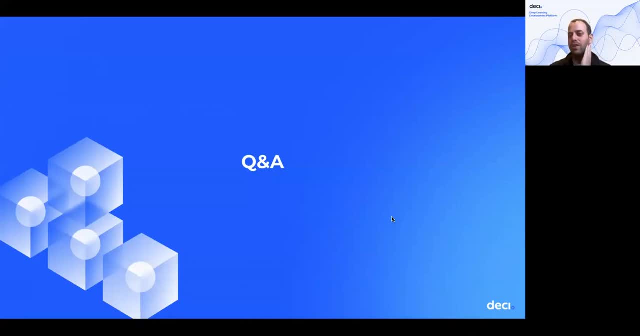 all evaluation metrics, that that everyone will agree on and that's really an open question. last week there was a significant change in in the open llm leaderboard, uh, that one of the data sets that called drop have been removed. um, so, uh, because of some uh differences in the evaluation results, 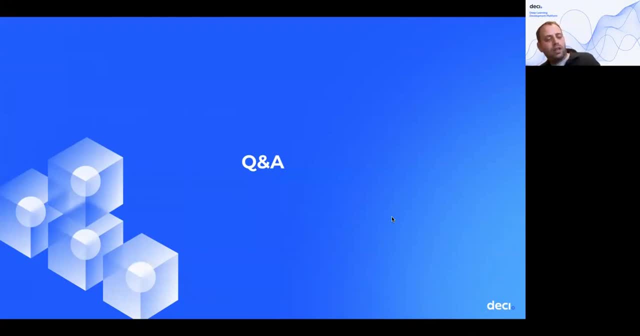 and things like that. so basically, how to evaluate uh, um an llm is is a good question, but what i recommend is first kind of eyeballing the, the results. uh, you can never trust numbers. we, during the development of of the clm7b, we had a version that we really liked um, and it has very 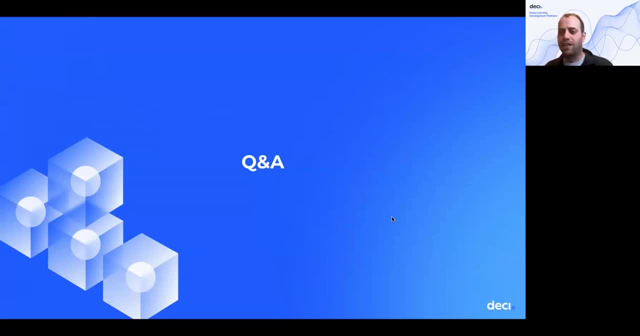 very good numbers on on all the llm eval numbers. but then when we started to to to play with the model, we saw that it behaves very weird and so in some uh, magical way it passed, like with very high scores, all all the numbers. so first thing to do is to play with the 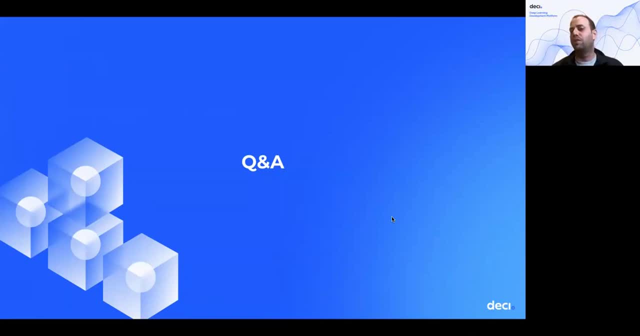 model. second thing is to go to all those model eval uh data sets and choose what tasks and what tests are best representing what i'm going to use uh for for my model, for example, the evaluation data set and and tasks for long context. if you're using the model for long context, uh, zero, short or 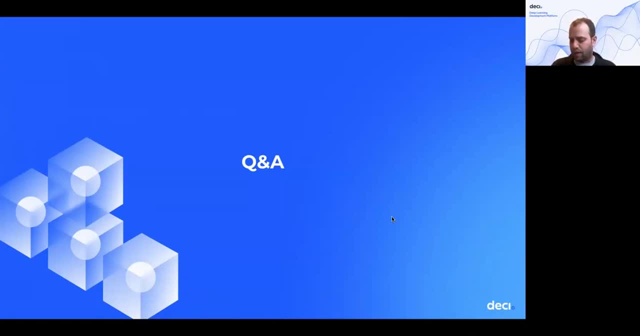 one shot, um that you should test that. if you're using for summarization, there's tests today to test on specifically on summarization. if you want to uh test the hallucinations, the tests today that test the hallucinations. so, basically, what i recommend is to to go through all the evaluation and data. 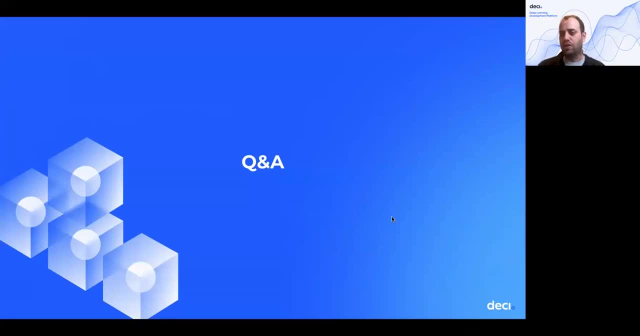 sets and the evals. those have been published on llms and choose like, pick which are the ones that you are mostly interested in. for example, if you are interested in math, there's the gsm uh test in the open llm leaderboard. that that is measuring. 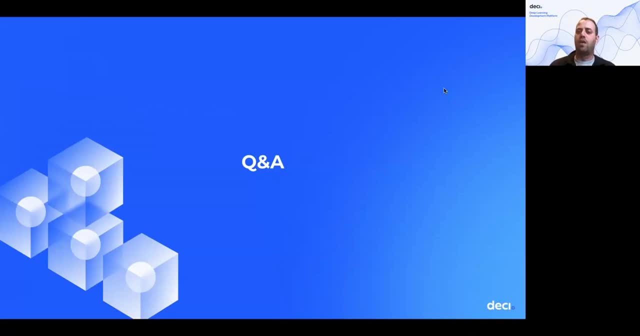 um, specifically this. so you should choose, uh, what benchmarks and what uh test cases you you should use for your um, for your uh, llm, um. so what are the uh aws? uh, how did we calculate the aws prices? um charge by the hour and context window. so it will. if i will go back to this slide, 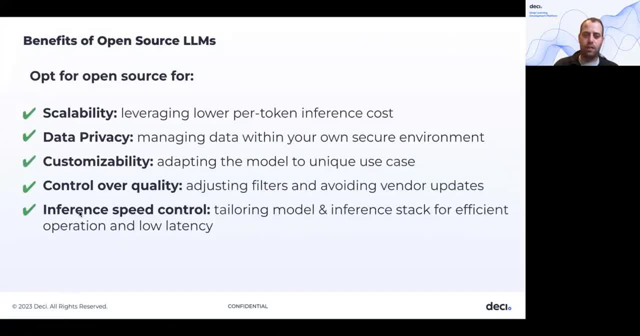 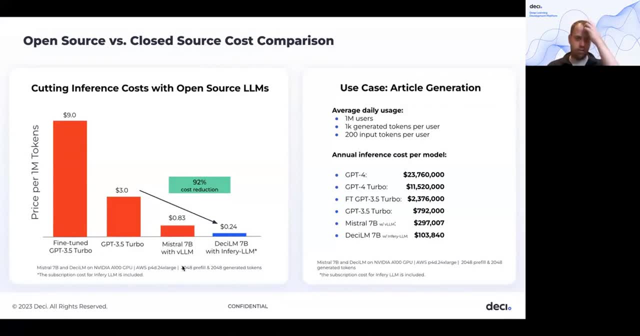 that we did the calculation with aws. there's some comments here, uh, below. so usually what we're doing for evaluation is that we're using same number of pre-fill, like context and generated tokens. um, so this is how we calculate the cost of the closed source models. but we're going to show you how to calculate the cost of the closed source models. 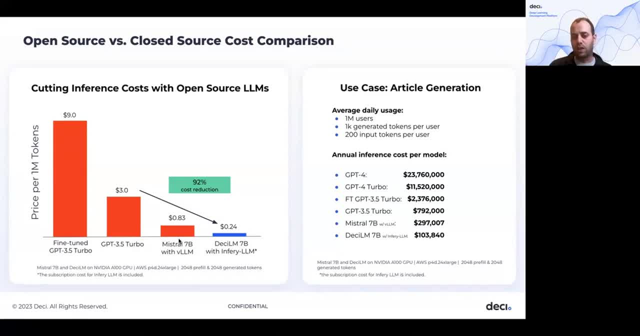 But also this is the performance benchmarks that we are doing for the open source models. Usually, the numbers that we are putting here, if I'm not mistaken, it's one year reserve pricing of AWS for machines In the A100, usually we take the price of the eight GPUs for A100 and divide it by eight to understand the cost of the benchmarks of one machine through one GPU. 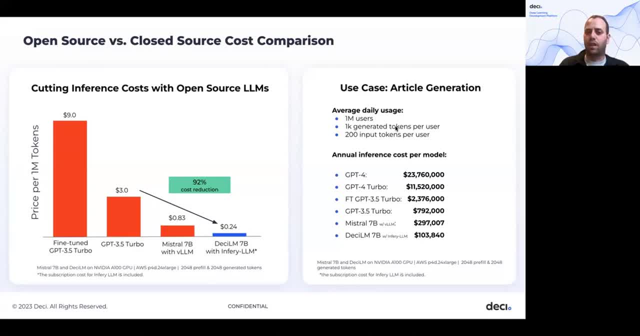 And obviously we can scale that linearly with Inferi LLM. So that's the way that we are calculating the cost And obviously when we are doing this calculation here on the right, we are adding the Inferi subscription, which is: 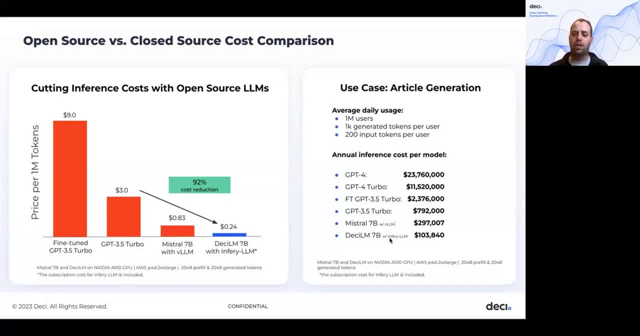 This is correlated with the number of GPU hours, so it's easy to add it here, and we still see that these numbers remain significantly lower than using open source VLLM and the Mistral model. But everything that computed here in terms of pricing of AWS use the same benchmark mechanism in terms of input and output. 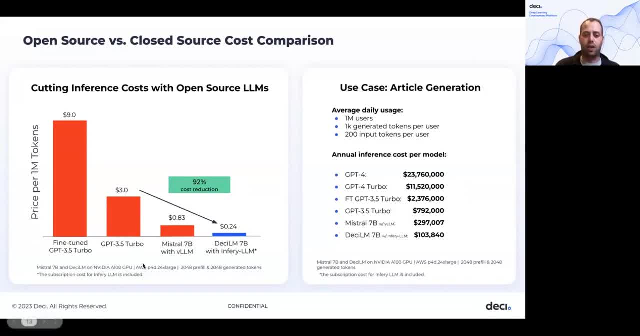 So we can see that the A100 has the same output sequence length. the same machine that we can see here, that's the A100 GPU- and the same one year reserve prices. I see here questions about converting PDF documents to question and answers. 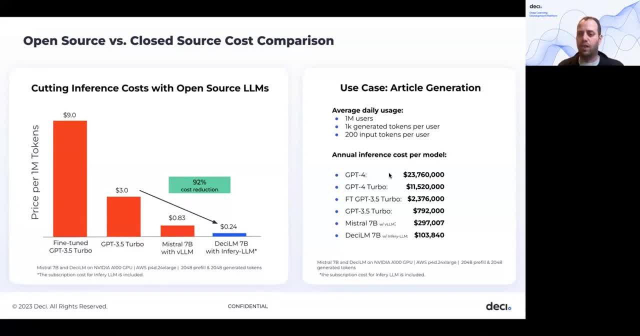 So using GPT for Turbo API. so it really depends on the length. but the CLM7B that we're releasing very, very soon is going to have a very long generation length. So basically, when we release it you'll see that you can feed documents and do kind of question answering on top of PDFs. 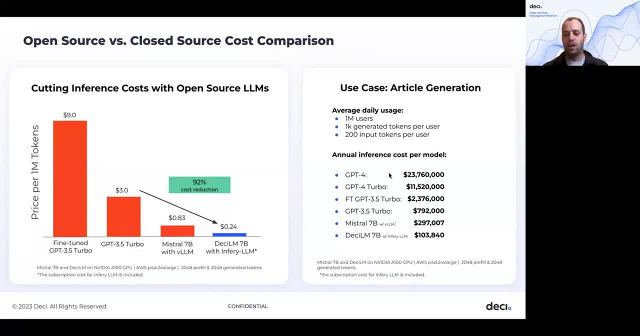 So I don't think that it will get to GPT for Turbo in terms of the context, but it really depends on how long the PDFs that you are trying to do. question answer. One of the things that we measured before we're going to launch that is that it behaves good with long context. 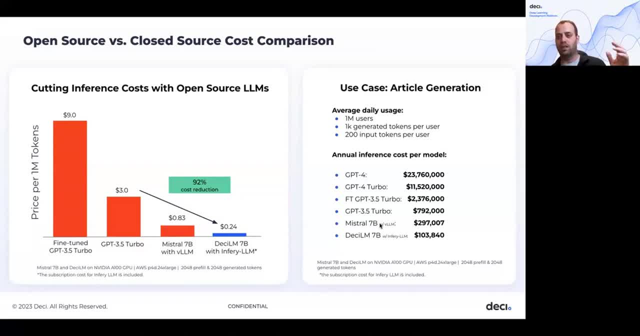 So there's a lot of question is whether models that promote that they have long context really support or memorize the long context. And since we trained it with did the pre-training with relatively long context lengths and we checked it and it's also memorize or digest that context length. 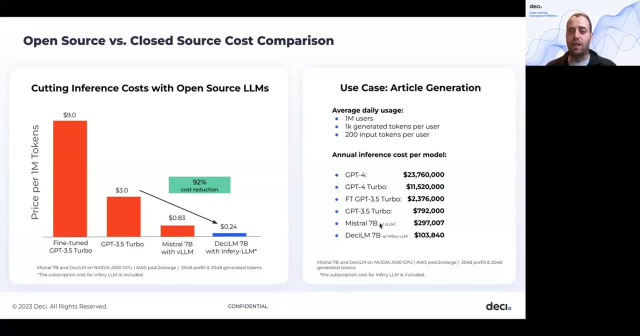 So you can use the CLM7B once it will be out and we'll be happy to hear your feedback about that In terms of API for PDF documents. so we don't have APIs, But we can give some tools to run it on your premise and maybe in the future we'll have some APIs to run those. open source and closed source. we answer that question. 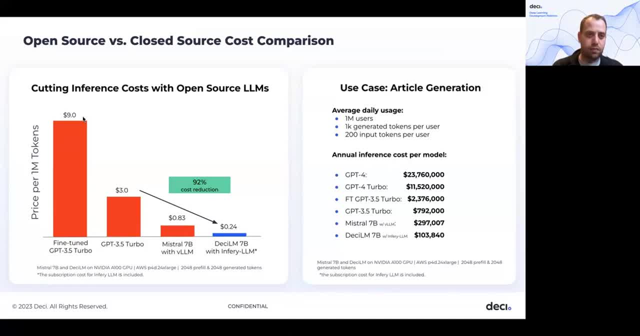 Let me see if I didn't miss any other question. I see people posting here some frameworks for evaluation of LLMs like Liquid, So that's a good answer. So for some of the questions that people ask you, I see a question about if the recording session will be available. 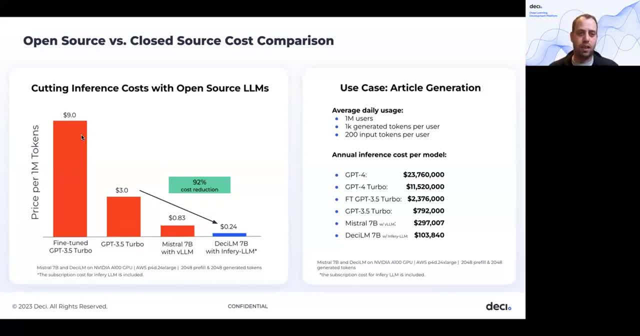 Yes, so you will get that recording. it will be available in the SCAI website slash resources, And I think that you will also get a link to the recording via a follow up email that will automatically be sent. So there is a question about- I think it's about- the code model, about its accuracy. 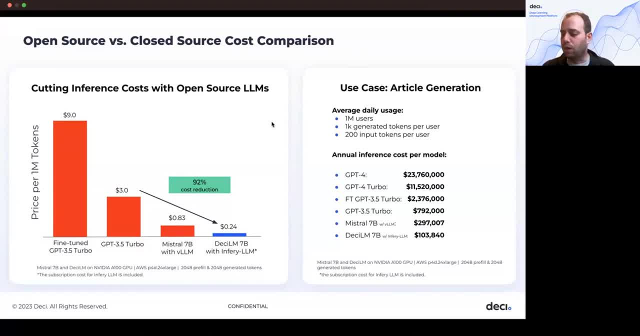 And one of the questions there about accuracy- that is below 20%. So it's really depends on the application. we need to understand how human evolved. Basically, it's a test that you get task and you complete the code and if the code running and passing tests, it's a hit and if not it's a loss. 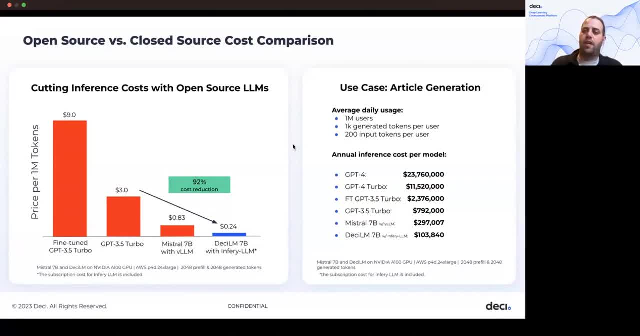 So that's an end to end task, But if you're using the model for code completion, the performance or the accuracy that you're going to do- in short, completion- are going to be much better than the 20%. Another thing to improve those models is: 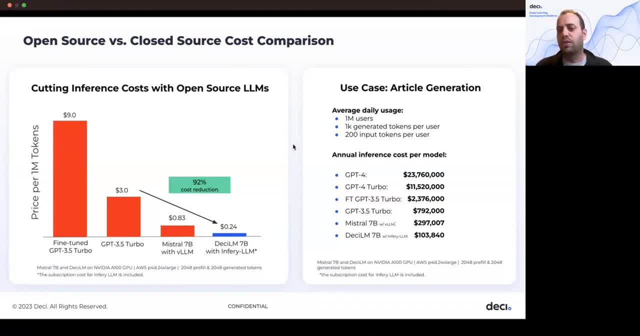 Fine tuning them to a specific programming languages. So those models are generalized in the sense that they know several programming language And if you want to do only Python, for example, you can fine tune the model to get specialized on Python. Another thing that we see companies are doing is fine tuning on their own code base. 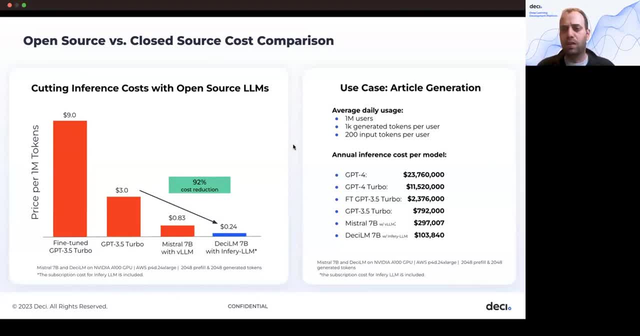 So then it can complete like calling to internal tools and functions and libraries. That's another cool thing that companies are doing In order to tailor even more code assistance systems in internal organizations. So that's another thing that we see that can be done. 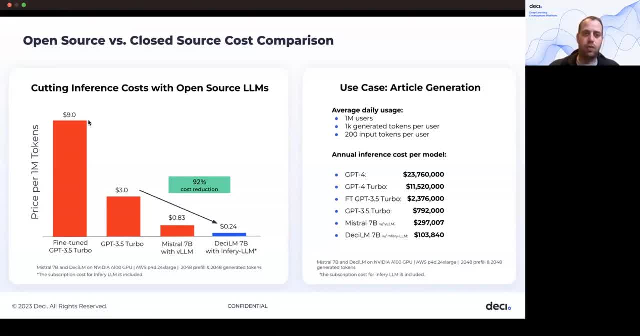 Yeah, so the last comment here is that the CLM will be on Hugging Face under Apache 2.0 license in a couple of days from now, And you can follow up on LinkedIn and get the updates when it will be out. Thank you very much for all the questions and the participation.